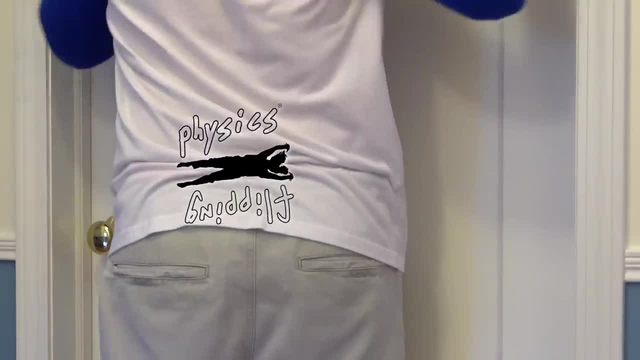 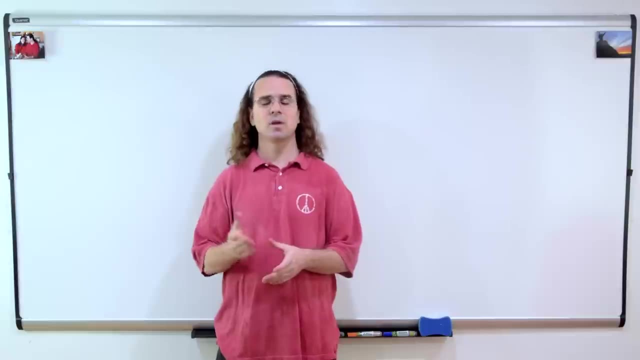 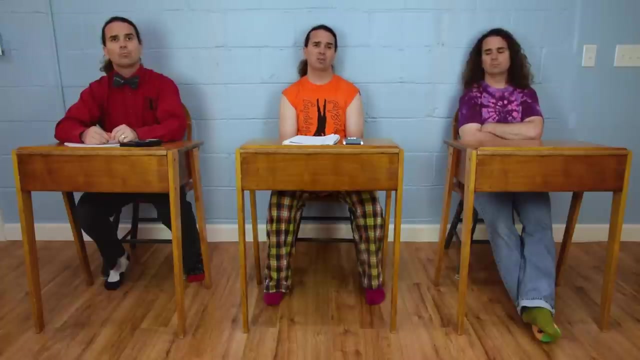 Good morning. Let's learn about torque Flipping Physics, But before we do, we need to review translational and rotational motion. Bobby, what is translational motion? Translational motion is like when something moves from one place to another right. 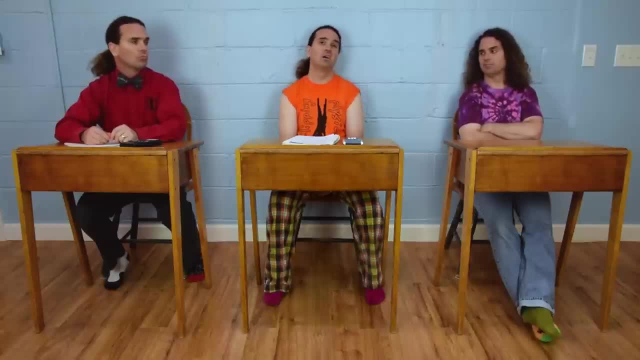 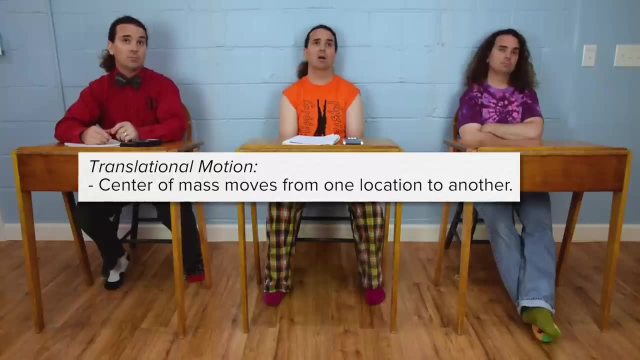 I think we need to refer to the center of mass of the object. Yeah, Uh, so translational motion is when the center of mass of an object moves from one place to another, And rotational motion is when the object moves in circles around its center of mass. 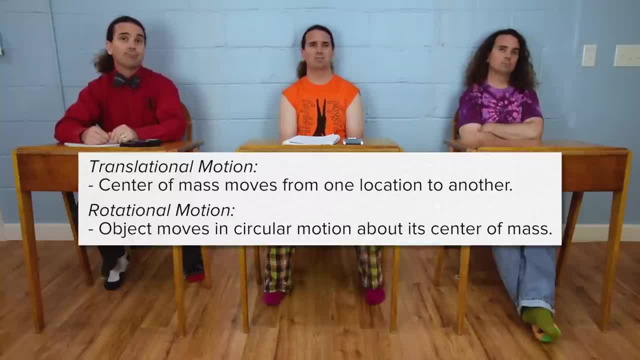 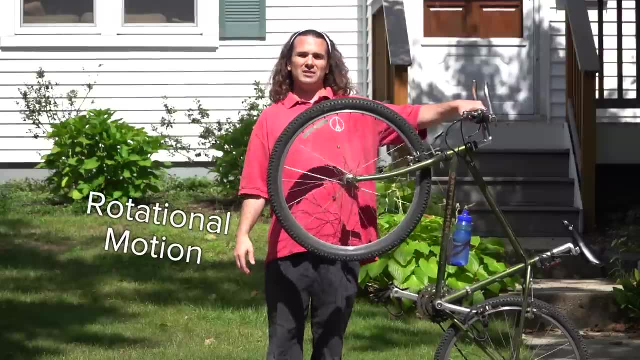 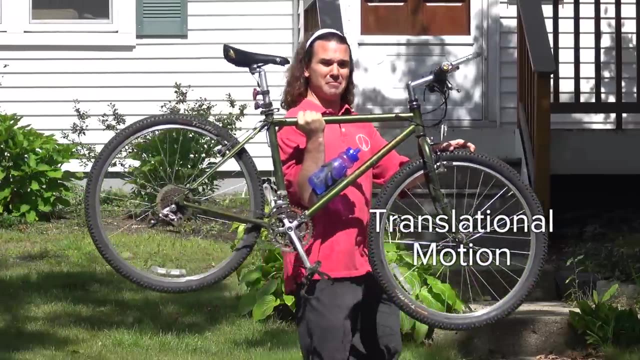 An object could have both translational and rotational motion. right, You are correct. Let's show some examples. This bicycle wheel is in rotational motion, but not translational motion. This bicycle wheel is in translational motion because its center of mass is in motion. 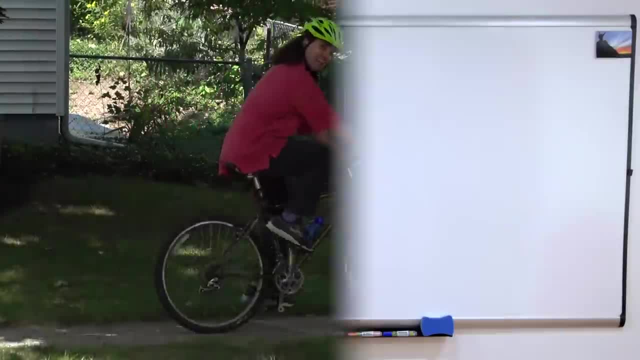 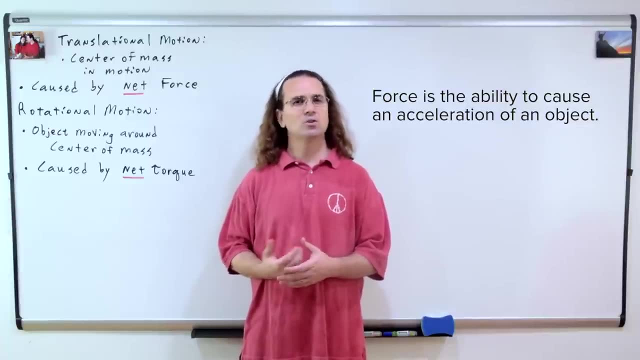 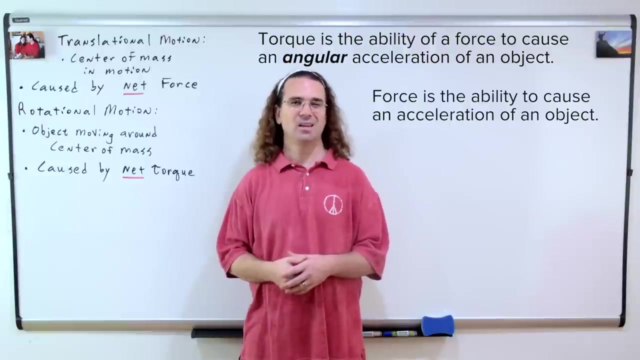 This bicycle wheel is in both translational and rotational motion. As you recall, force is the ability to cause acceleration. Well, torque is essentially rotational force. It is the ability of a force to cause angular acceleration. Watch as I apply a torque to a bicycle wheel twice. 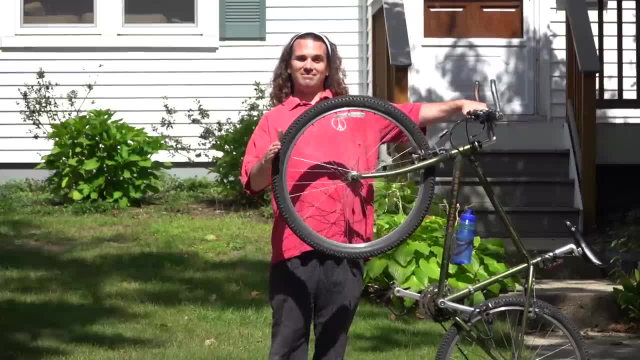 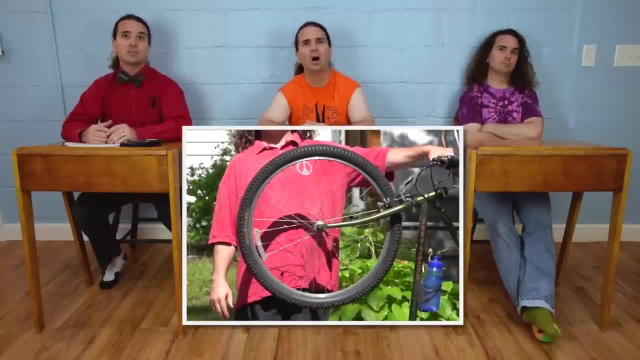 Billy, please explain how it is that you know I applied a net torque to the bicycle wheel twice. First the wheel was at rest, Then you started the wheel spinning, so you changed the angular velocity of the wheel. That means you angularly accelerated the wheel. 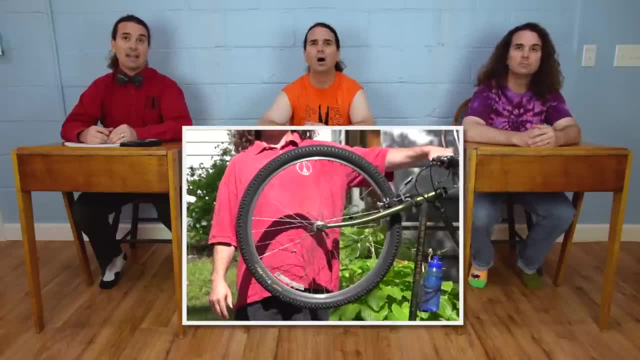 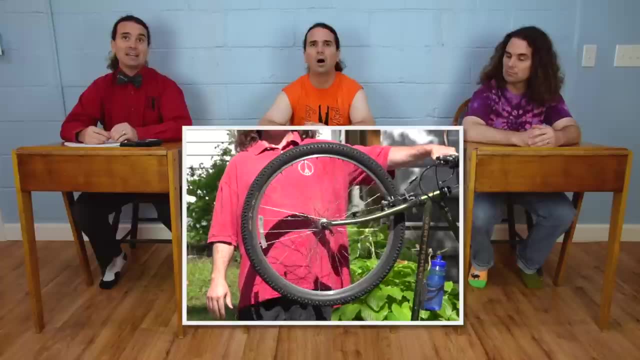 which means you applied a net torque to the wheel to cause that angular acceleration. Then you did the reverse: The wheel was spinning and you stopped it. So again you applied a net torque to the wheel to angularly accelerate the wheel. You changed the angular velocity of the wheel to zero. 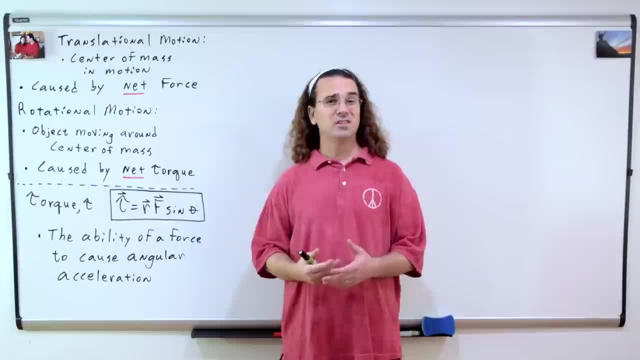 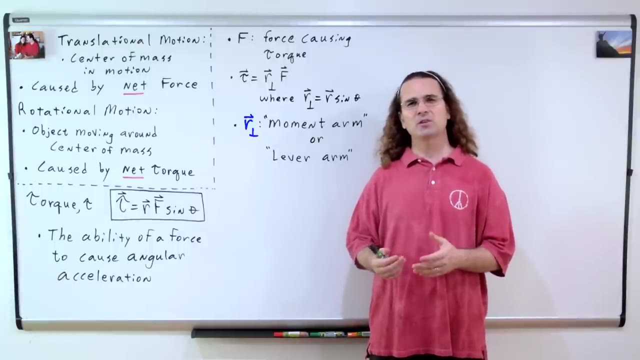 Billy, that's very nice. The symbol for torque is the lowercase Greek letter tau. It looks like a curly T And torque equals rf sine theta. F is the force causing the torque. This r perpendicular is called either the moment arm or the lever arm, and it equals r times sine theta. This means that sometimes the equation 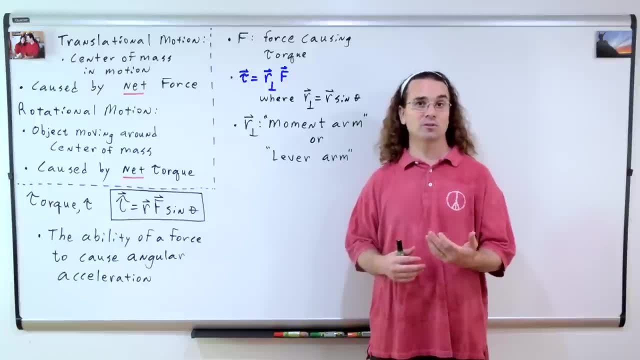 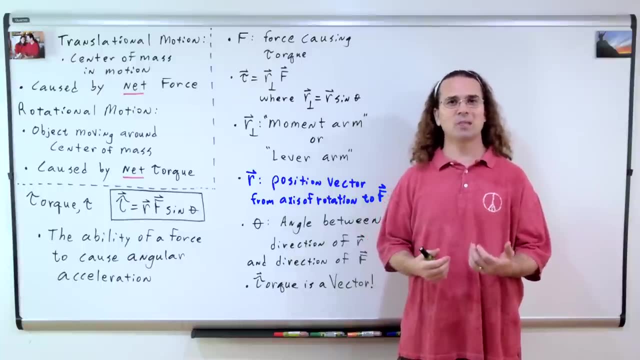 for torque is given as the moment arm times the force. The r vector is the position vector: from the axis of rotation to the point the force is applied to the wheel. The r vector is the position vector: from the axis of rotation to the point the force is applied to the wheel. 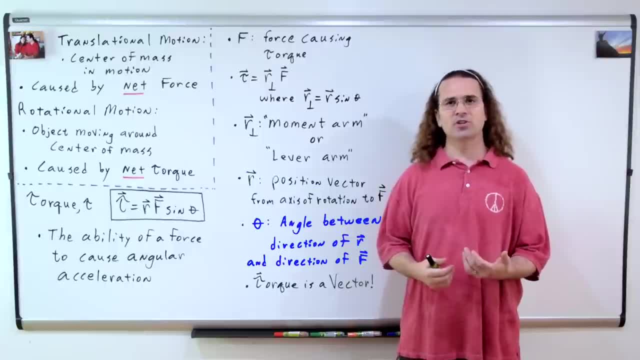 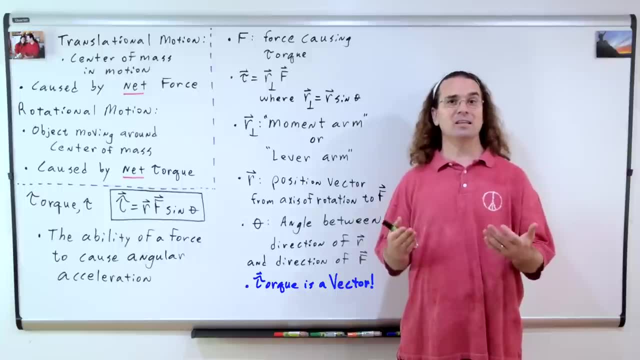 The r vector is the position vector from the axis of rotation to the point the force is applied to the wheel, And theta is the angle between the direction of the r vector and the direction of the force vector. And the arrow symbol over tau means torque is a vector. 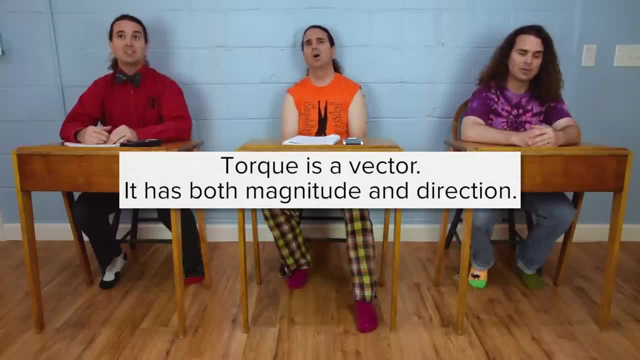 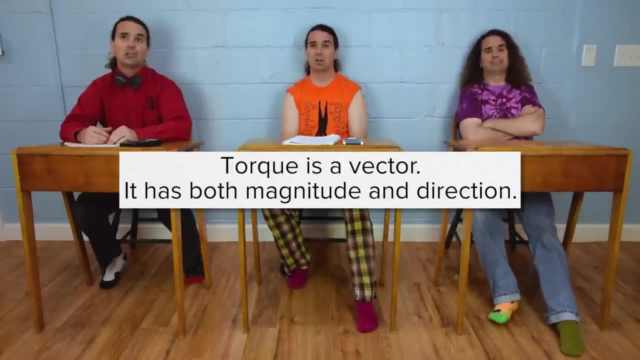 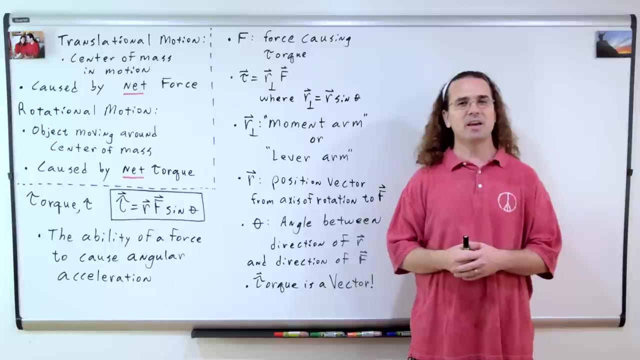 which means class torque has both magnitude and direction. That's great, but I have no idea what you were talking about with that r vector moment, arm lever thing. Right, There is a lot here. So let's look at some specific examples to help us understand. 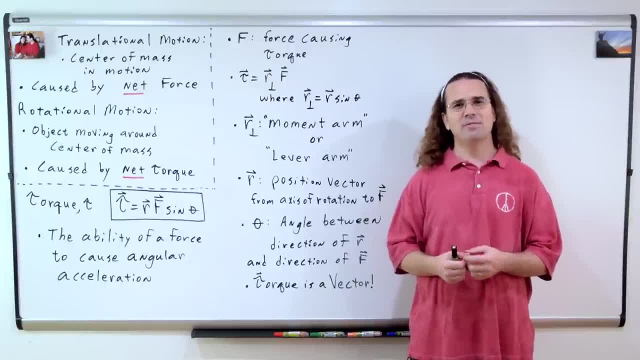 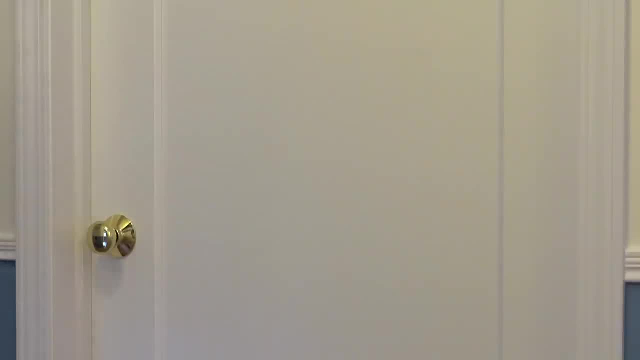 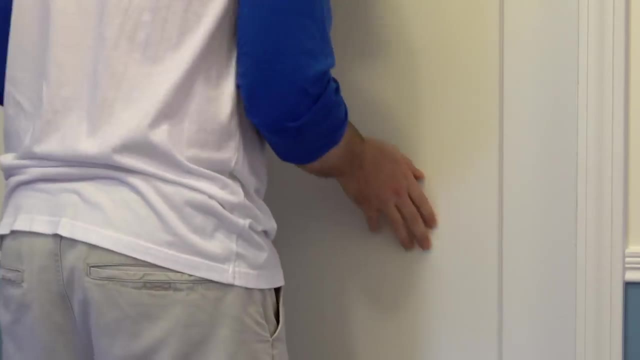 all of this, I'd like to say everything you ever needed to know about torque. you already know because you have opened many doors, So let's look at a door. Through trial and error, you have honed your ability to walk through a door. When you approach a door class, what do you look for? 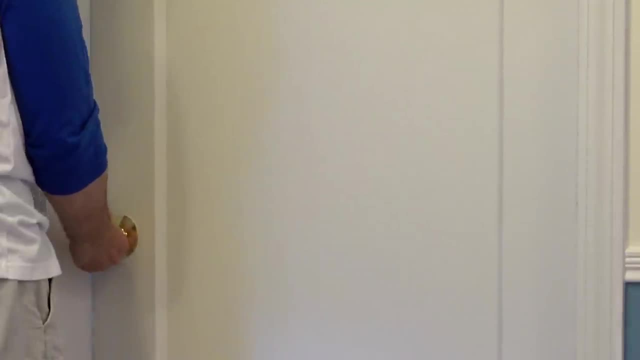 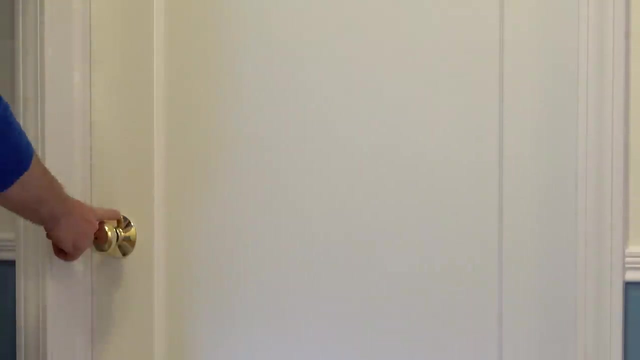 The handle And the handle is located where relative to the hinge, which is the axis of rotation. The handle is far away from the hinge Right. The handle is far away from the hinge. The handle of the door is about as far away from the axis of rotation or hinge. 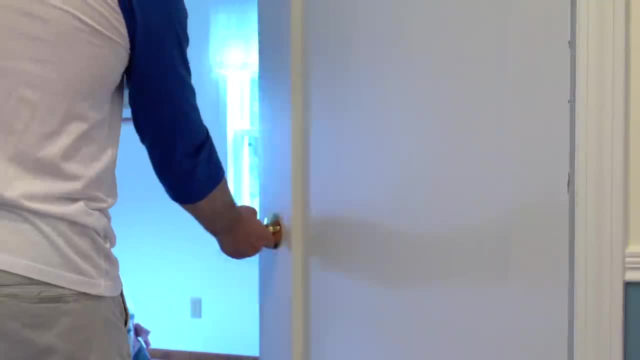 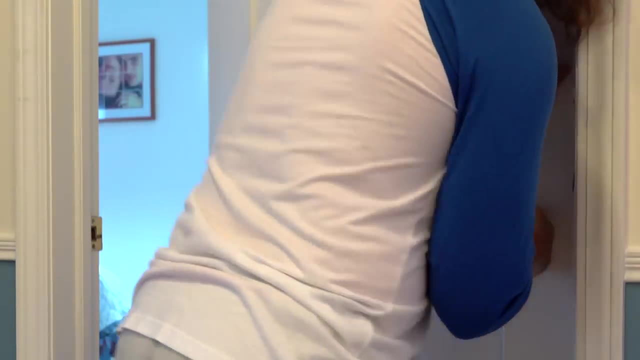 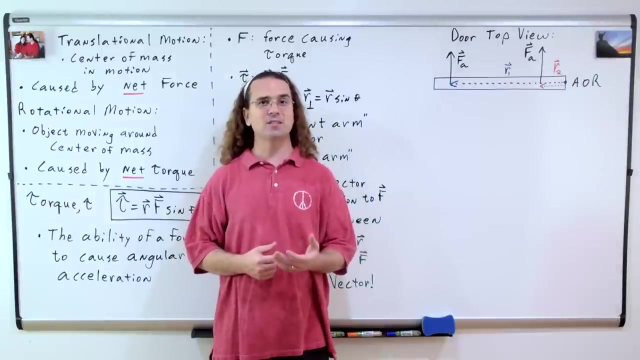 as the handle can get on the door. When you open a door, you push near the handle. You have learned not to try to open the door by pushing near the hinge, or axis of rotation. Let's talk about why that is. The magnitude of the r value is from the axis of rotation to where the force is applied. 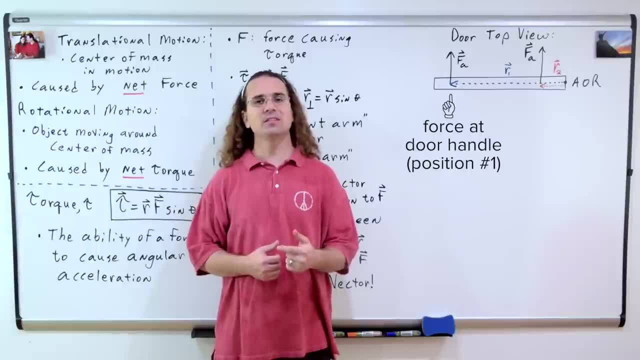 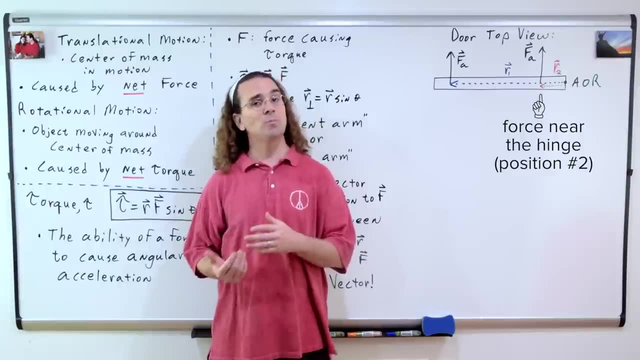 So when we apply a force at the door handle, there is a larger r value- r1, than if we apply a force near the axis of rotation, which has a smaller r value- r2.. If the force applied has the same magnitude and direction, 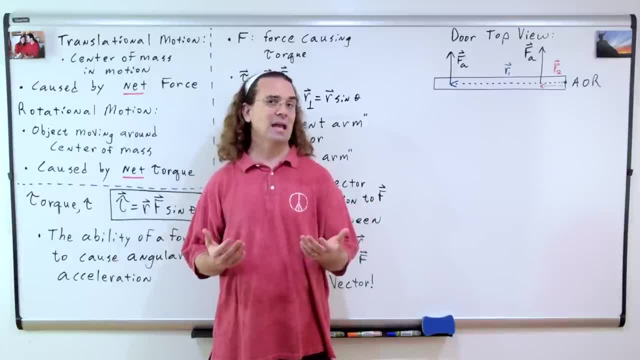 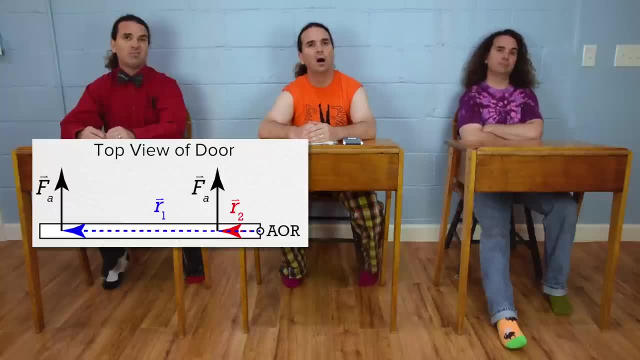 Billy, how do the torques compare at positions 1 and 2?? Well, it looks like the angle between the force direction and the r vector for both positions are 90 degrees, and the sine of 90 degrees equals 1.. So the torque in this case is just the r value. 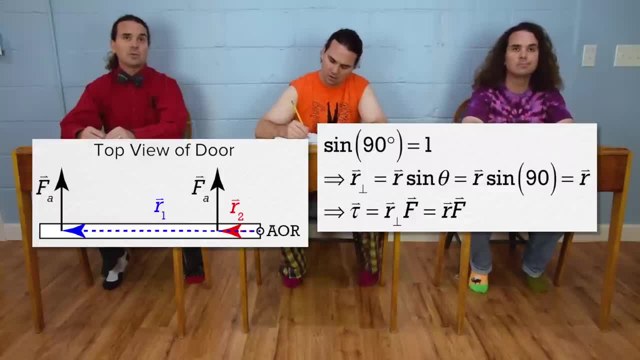 force applied Because the r value for position 2 is so much smaller than the r value for position 1, the torque when we push on the door closer to the axis of rotation is much smaller. And what does that mean for being able to open the door? 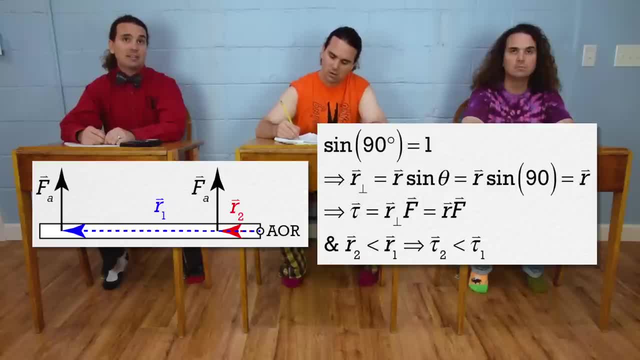 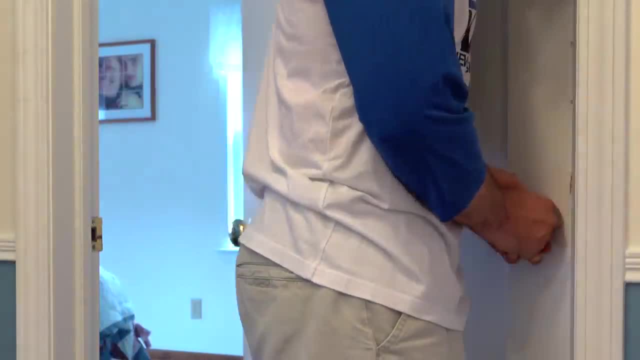 A smaller torque means a smaller ability to cause an angular acceleration. So when we push near the hinge the torque has a smaller ability to cause an angular acceleration to open the door. Absolutely, Billy. thank you. Another thing we have to know about the angle between the door and the 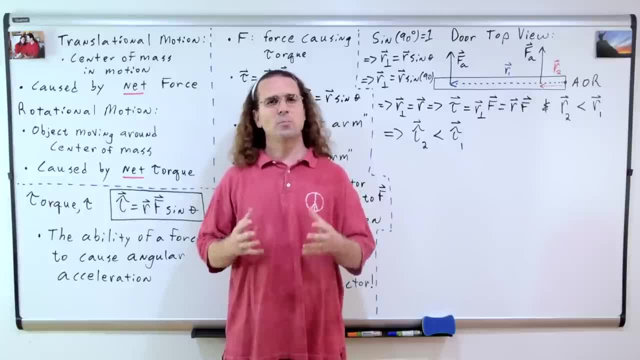 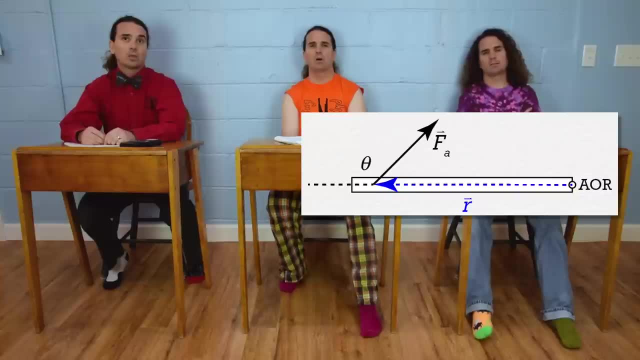 hammer is that we have to learn to never do. to try to open a door is to push at an angle like this. Bobby, why will we never try to open a door by pushing at an angle like this? Okay, so when we push at an angle that's not 90 degrees, oh, 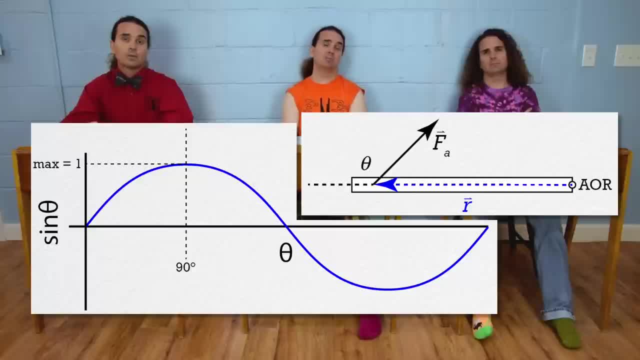 because the shape of the sine curve is, the maximum value for the sine of an angle is at 90 degrees. So at an angle that is not 90 degrees, the sine of the angle, the sine of the angle, will be less, which will make the door class, which means the ability to cause an angular acceleration to open the door, is less. 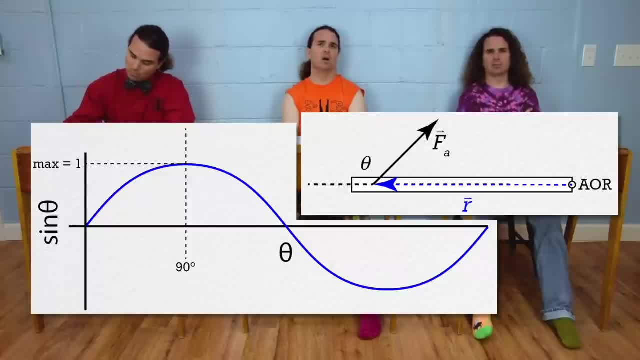 Why is the angle theta on that side of the force? I thought he said it was between the force and the r-vector. Oh, theta is between the direction of the force and the direction of the r-vector. The r-vector points to the left, so theta is between to the left and the direction of the force. 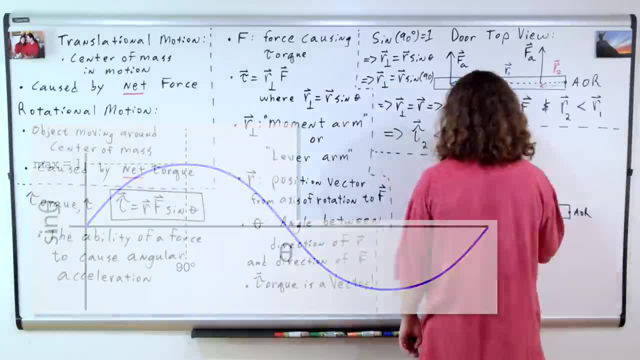 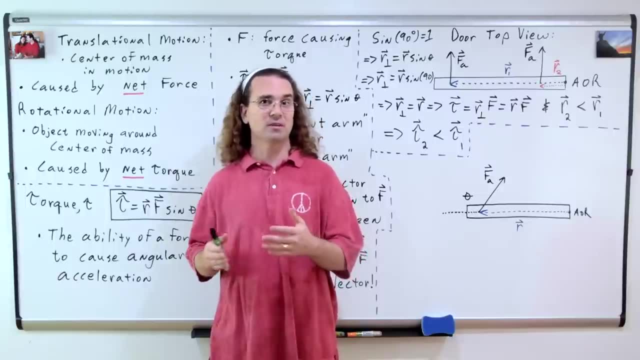 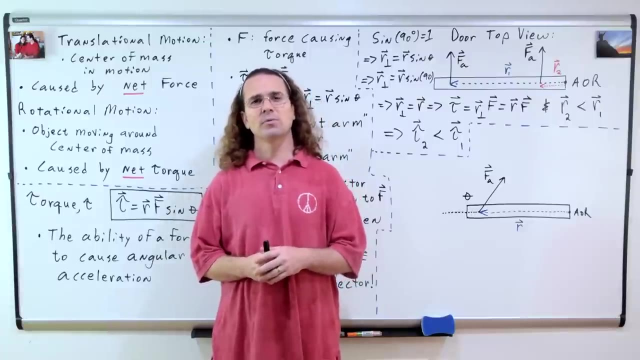 Okay, that makes sense. Thanks, You're welcome, Mrp. Very nice, Bobby, You are correct that because the sine of 90 degrees results in the maximum value for the sine of the angle, an angle of 90 degrees between the direction of the force vector and the direction of the r-vector will result in the maximum torque. 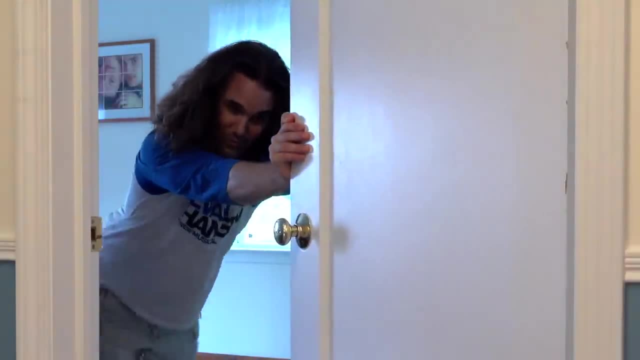 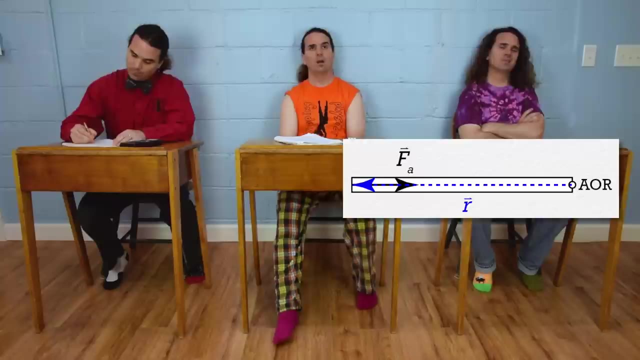 Okay, one last example of how you will never try to open a door, Bo. why will you never try to open a door by pushing on the side of the door like this? Well, in that case the angle between the r-vector and the force vector is less. 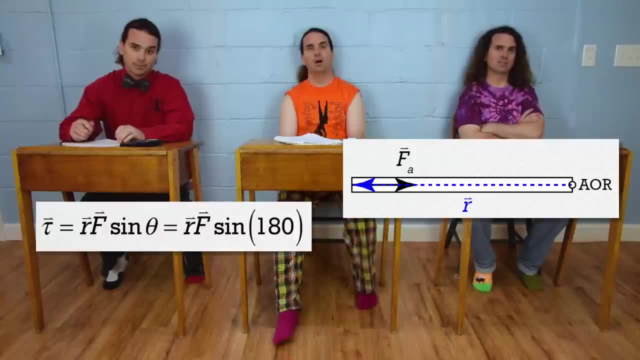 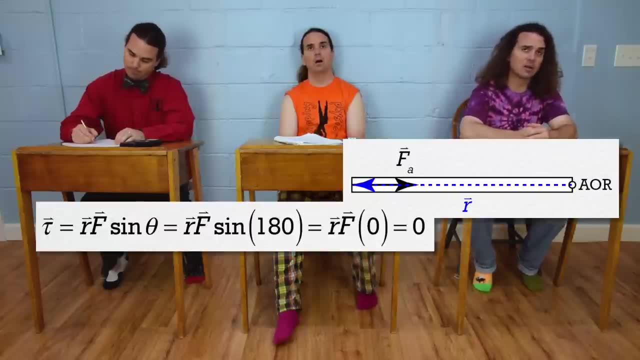 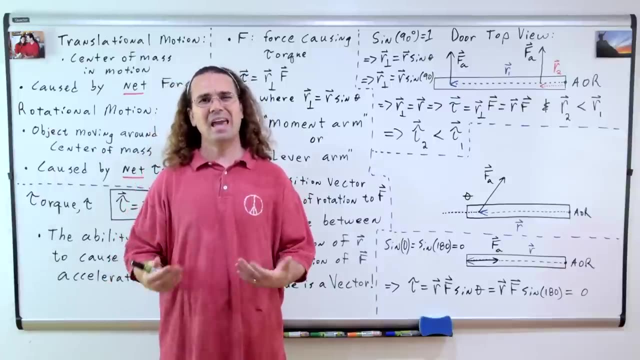 The r-value and the force applied is 180 degrees and the sine of 180 degrees is zero. So no matter how hard you push, that will never cause a torque on the door, Mrp, Correct. No matter how hard I push or even pull on the side of the door. 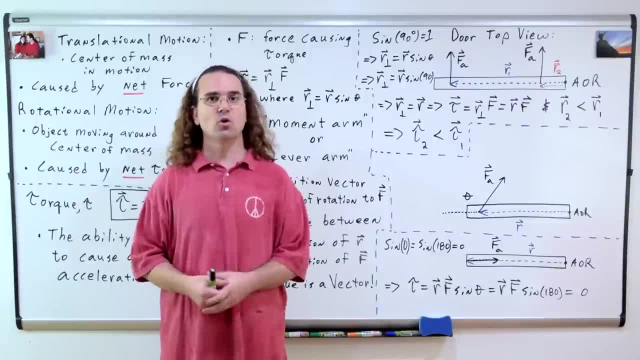 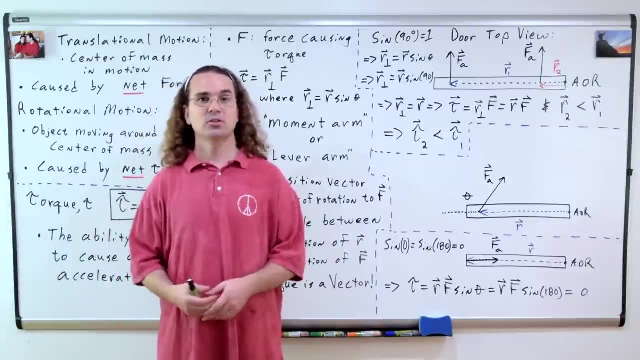 the angle will be either 180 degrees for a push or zero degrees for a pull, Regardless the sine of zero and 180 degrees are both zero, So there is no torque And no ability to cause an angular acceleration of the door. 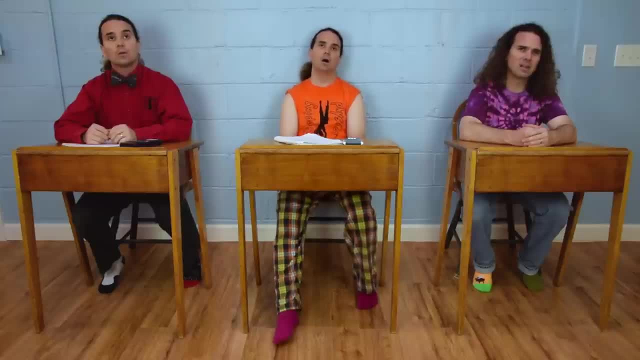 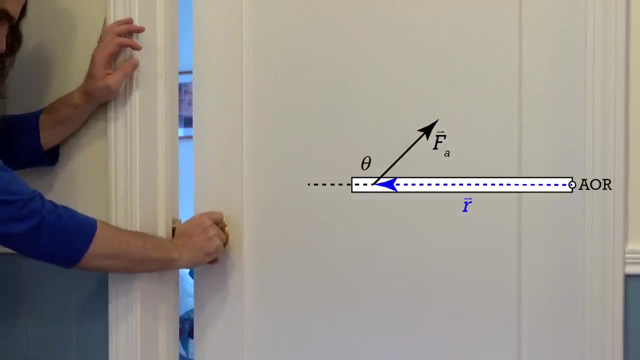 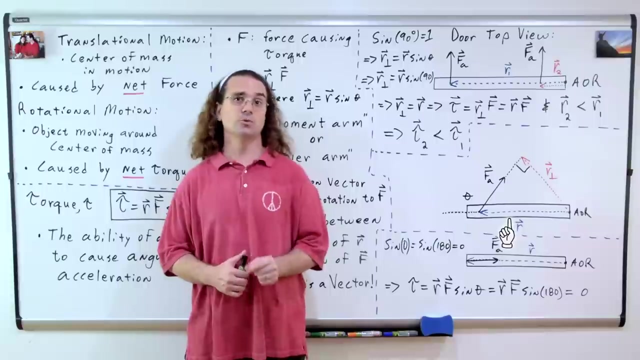 Mrp: Yes, Bo. What about moment arm or lever arm? You have not mentioned that at all, Mrp. Right, Let's go back to the example with the force at an angle to talk about the moment arm. The r-position vector is the hypotenuse of a right triangle which has two sides. 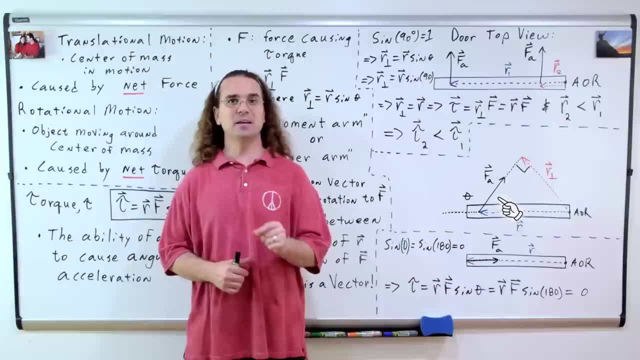 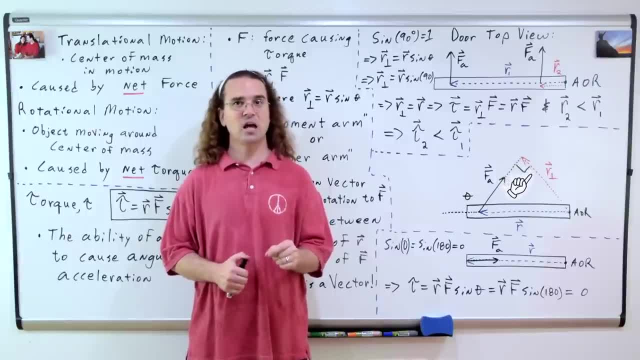 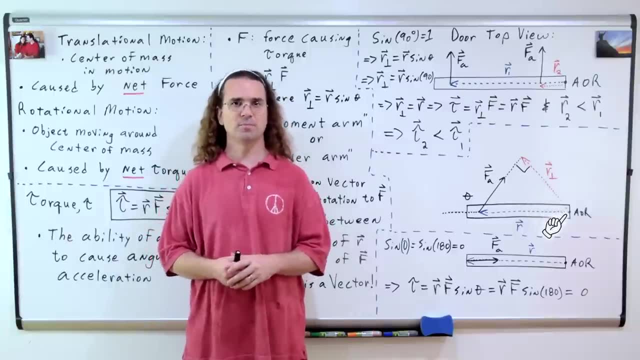 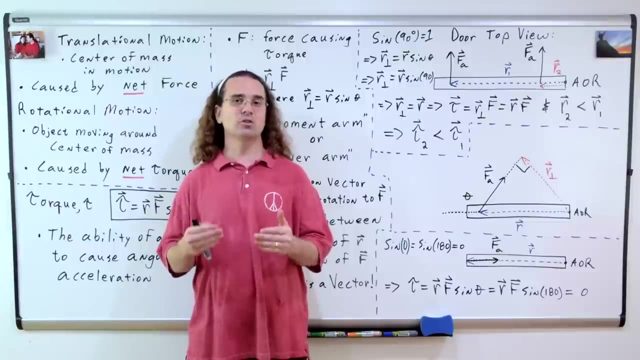 The other side is the component of the r-vector which is perpendicular to the extension line of the force. This perpendicular component of r is called the moment arm or the lever arm. Notice in this example that the moment arm is smaller than the r-vector because the angle in our torque equation is not 90 degrees. 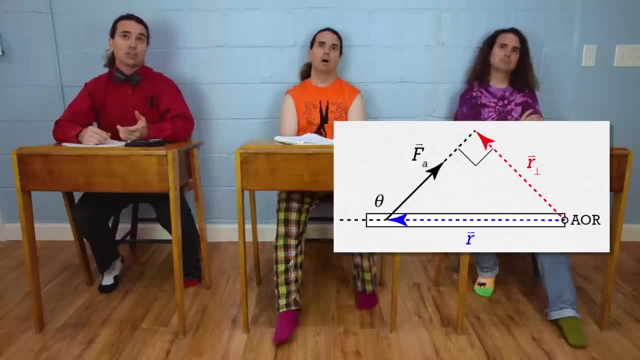 Oh, and when the angle is 90 degrees, like the first door example, the r-value and moment arm are equal in magnitude. And when the angle is 180 degrees, like in the last example where you pushed on the side of the door. 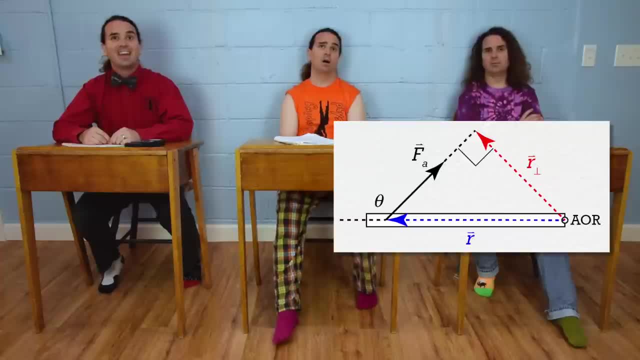 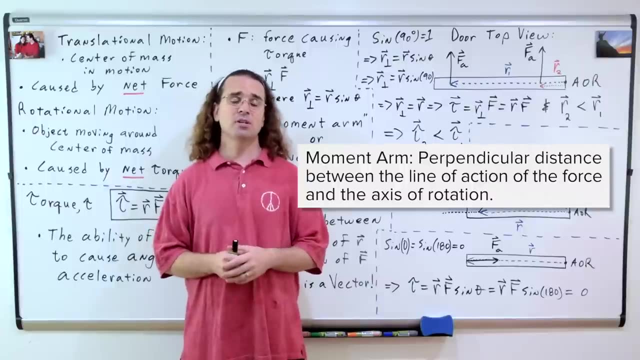 the moment arm is actually zero. I agree with all that, but that does not really explain what the moment arm is. Yeah, Right, Okay, The moment arm is defined as the perpendicular distance between the line of action of the force and the axis of rotation. 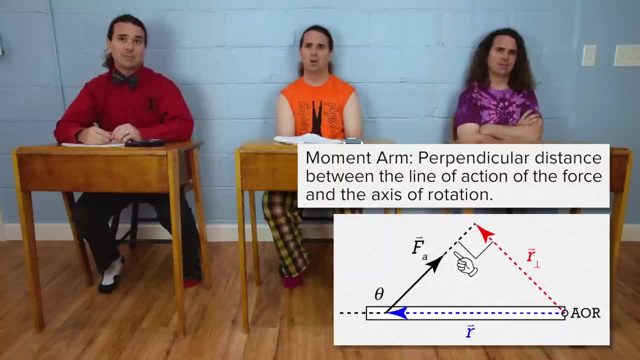 Right, Sure. So the dotted line extending from the force must be the line of action of the force, And the moment arm is the perpendicular distance between the line of action of the force and the axis of rotation. And the moment arm is the perpendicular distance from the axis of rotation to the line of action of the force. 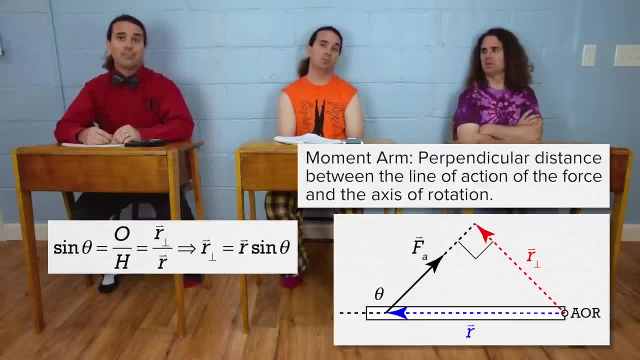 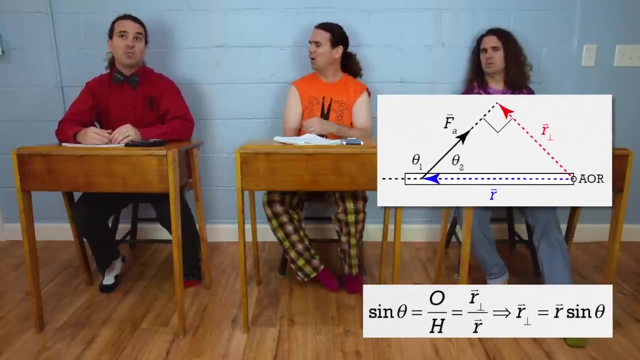 Perpendicular because it's a right triangle And sine of theta equals opposite over hypotenuse, or moment arm over r-value. So the moment arm equals r sine theta. I thought theta was on the other side, Right. Those two angles- let's call them theta 1 and theta 2, are supplementary angles.